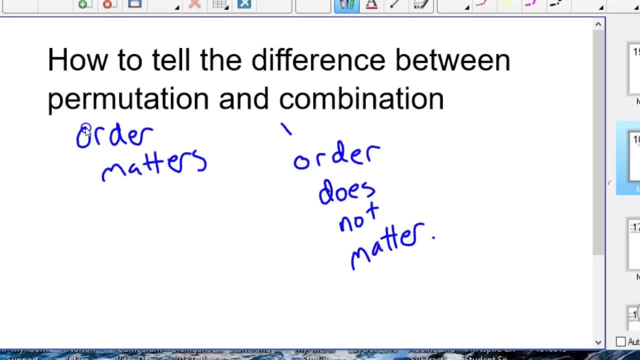 And essentially we have to make sure we don't count things twice. You should only count things once, And if we do everything as a permutation, you'll always overcount. So you've got to have two: a permutation and a combination. 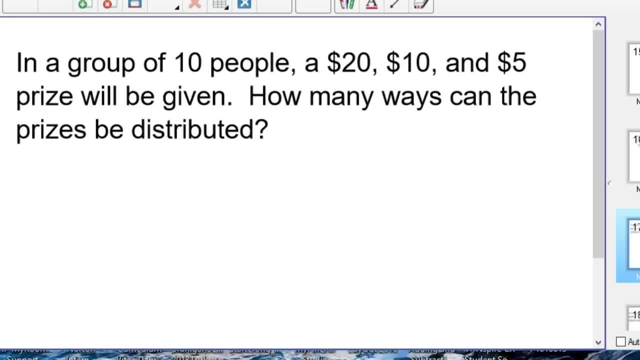 So here's the first one. It says, in a group of 10 people, a $20 bill, a $10 bill and a $5 bill prize will be given out. How many ways can the prizes be distributed? So hit pause on the video. 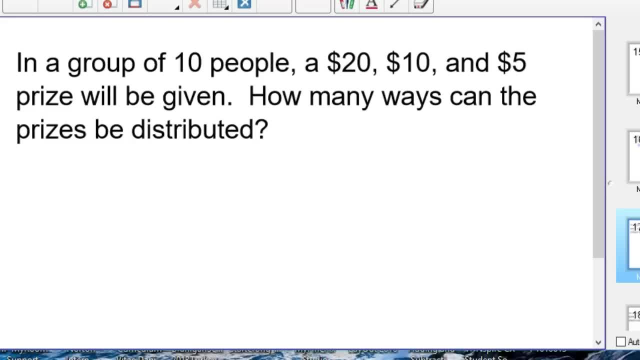 And see if you know which this is, And then try to solve it. Alright, This is a permutation, Because order matters. It matters who gets the $20.. It matters who gets the $10 and who gets the $5.. At least it's going to matter to them. 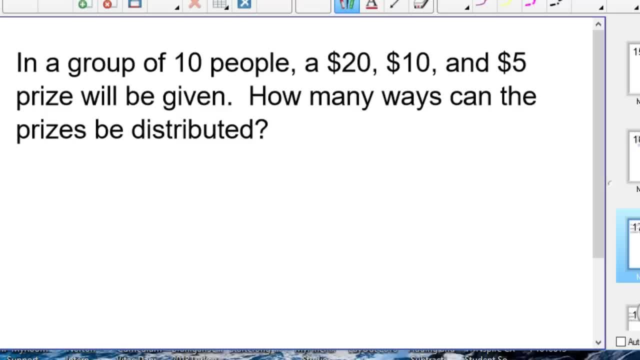 It may not matter to the person giving out the money, But it definitely matters to the people receiving the money. So this is a permutation, So we have three bins to fill, And I always like solving permutations this way. So there's 10 possibilities for the first person, for the first prize, for the $20 bill. 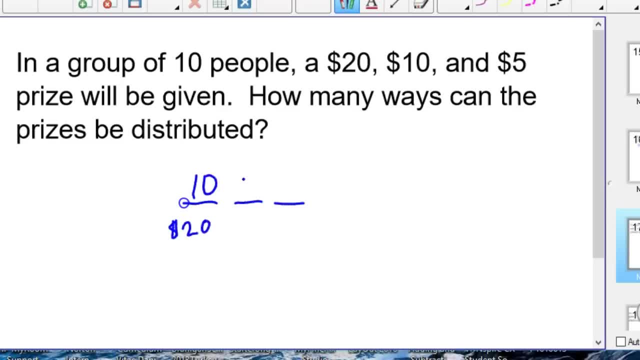 So this would be the $20 bill. There's 9 possibilities. I started writing the $10 bill there For the $10 bill. now we've chosen somebody for the $20.. Now we only have 9 possibilities for the $10. 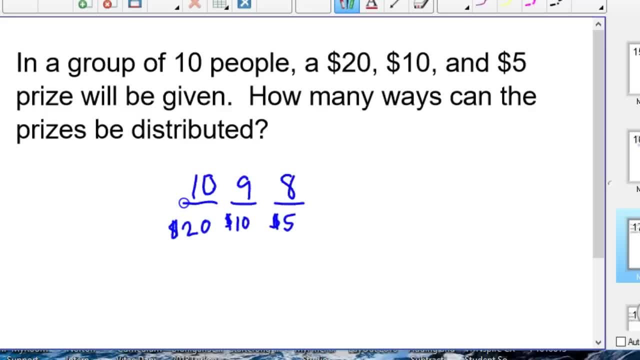 And for the $5 bill, we have 8 possibilities, And so this is this would be your answer- Or 720.. 10 times 9 times 8.. If you did it with the permutation formula, it would be 10P3. 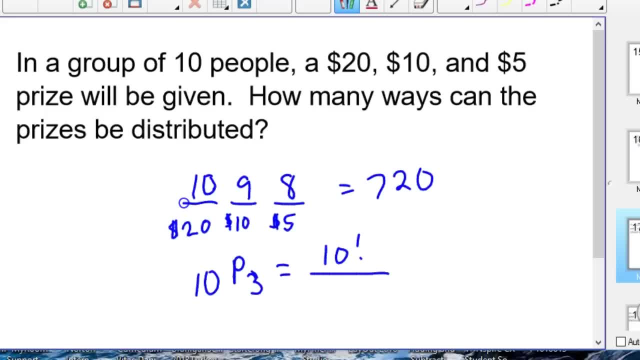 which would be 10 factorial divided by 10 minus 3, which is 7 factorial. And if you did that, 10, 9,, 8,, 7,, 6,, 5, 4, 3,, 2, 1, is 10 factorial. 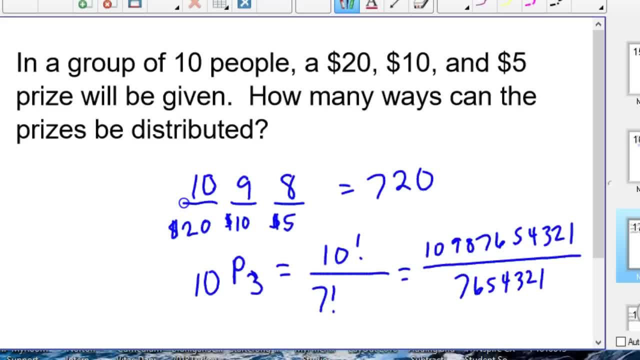 7, 6,, 5, 4, 3,, 2, 1, is 7 factorial. You could cross those out and you're left with 10 times 9 times 8.. So that's using the formula. 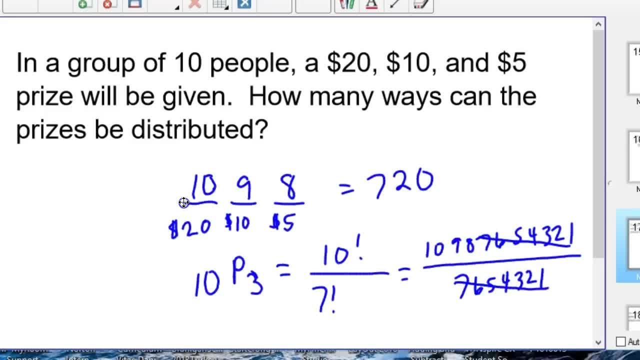 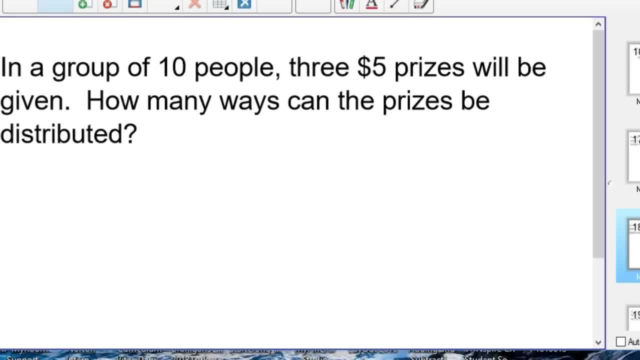 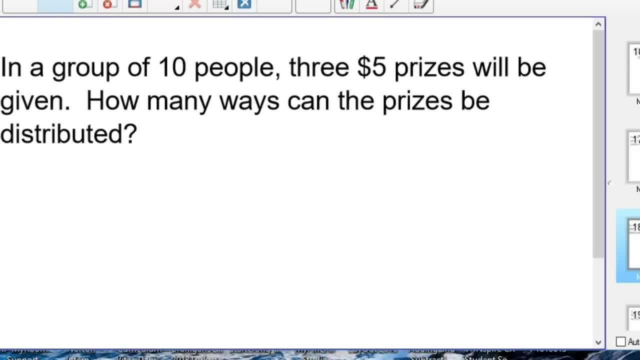 How many ways can the prize be distributed? So again, pause the video. see if you know what this is. It's probably pretty obvious, since I just did the other one, But go ahead and try and solve it and see if you know how to do it. 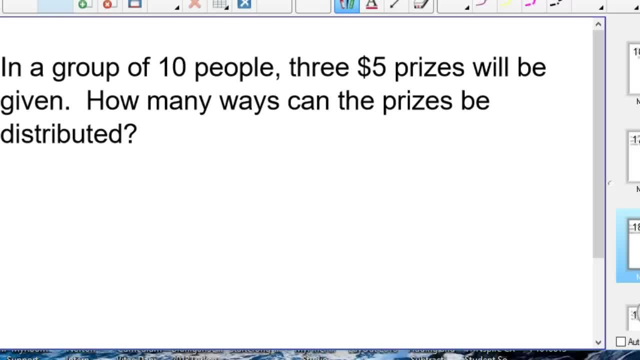 So, in this case, 10 people, we're going to do three prizes. Order does not matter, So we're going to go ahead and use a combination, which would be 10 choose 3.. So we're going to give out three prizes. 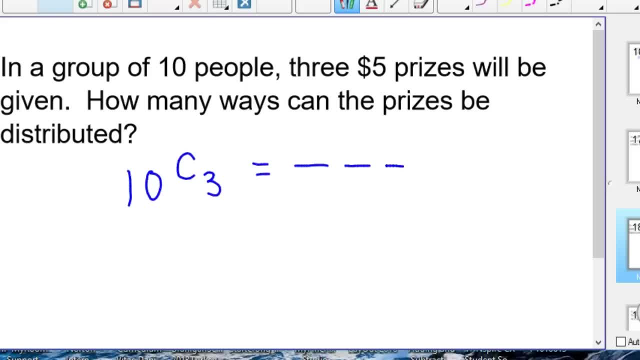 And so again, I like to solve this with the bins like a permutation, but then just divide out the repeating part. So there's 10 for the first $5 prize, If you've already chosen that, now there's only nine people. 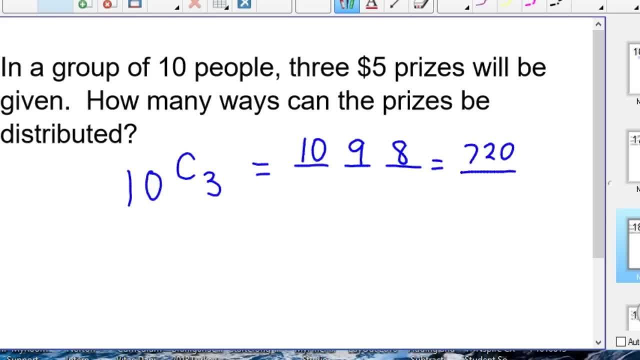 then eight people, which is 720.. However, we need to divide out. We've counted things twice, So we need to divide out three factorial- six ways of counting things twice. And so you're left with 120 this time, And if you look at the formula, it's 10 factorial divided by seven factorial. 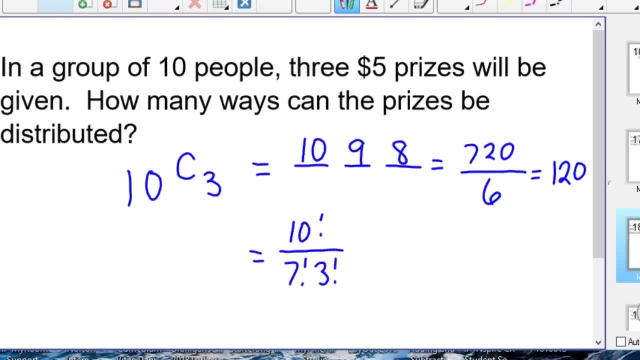 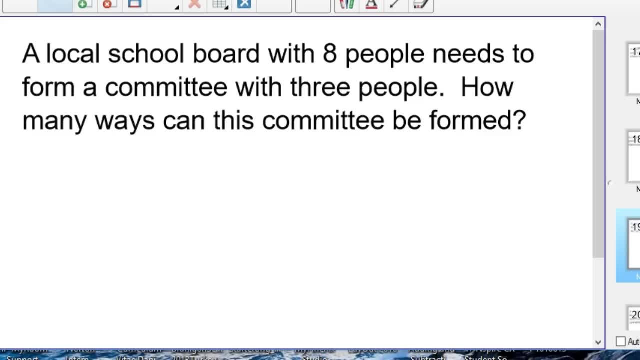 just like a permutation. but you'd also divide by three factorial And that gives you a 120.. I'm not going to go through the multiplication on that, So here's another one that's a different scenario: A local school board with eight people. 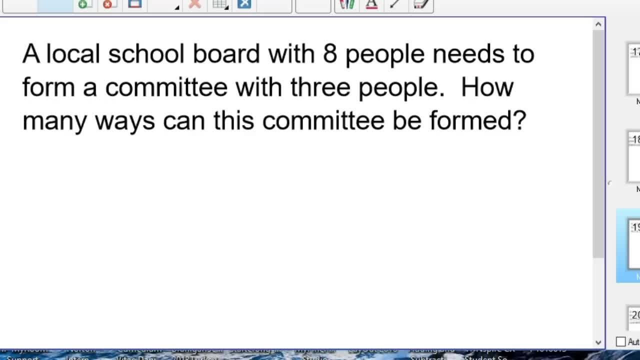 A local school board with eight people needs to form a committee with three people. How many ways can this committee be formed? So again, see if you know which one this is. Hit pause, try to solve it. So in this case, this is a combination. 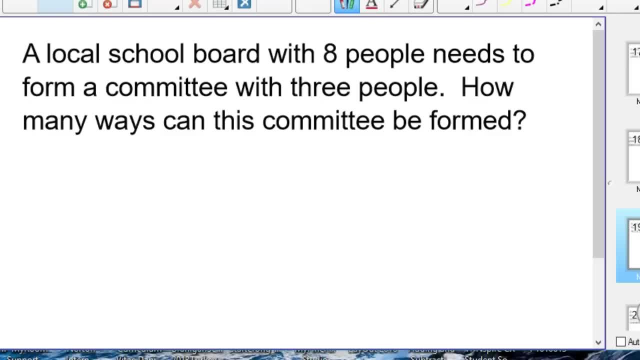 Order doesn't matter, They're a committee. They all have equal jobs to do in a committee. So we've got eight, choosing three, which would be eight factorial, divided by eight, minus three, which would be five factorial, also divided by three, factorial of what we're choosing. 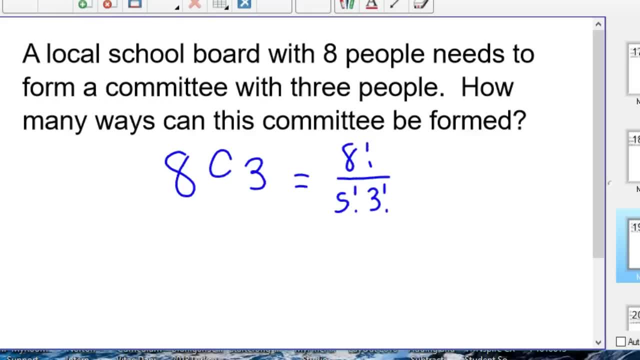 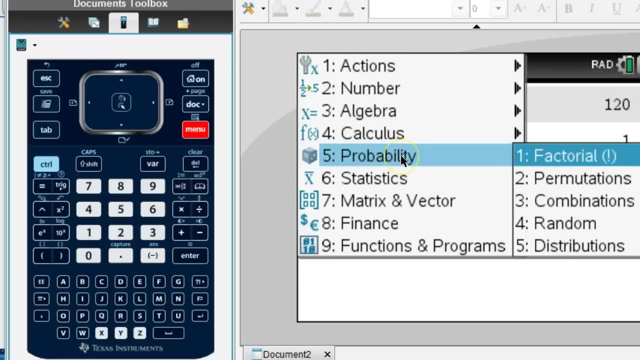 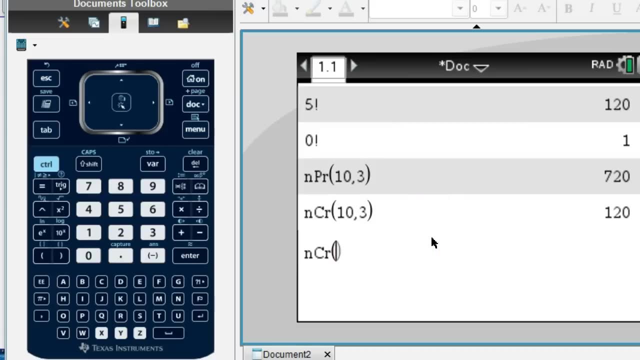 So this time I'll get out the TI Inspire calculator just to show you how to plug them in. So you'd hit menu probability. This is after hitting calculator. by the way, This is a combination, and it was eight. choose three. 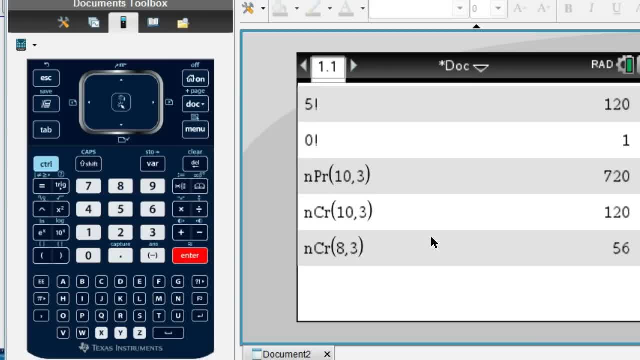 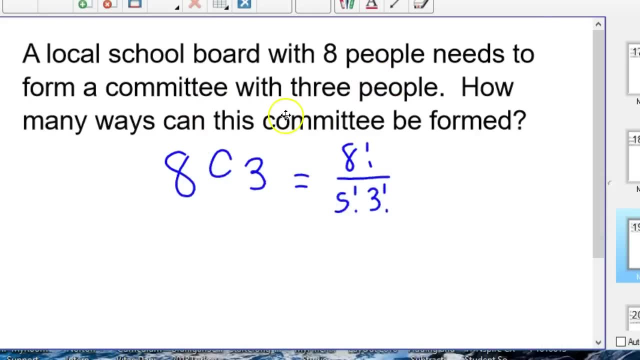 So there's eight. three Hit enter and that is 56. So there's 56 ways. If you have a school board with eight people, there's 56 ways to make a committee of three. So the next thing: let's see if we've got another problem on here. 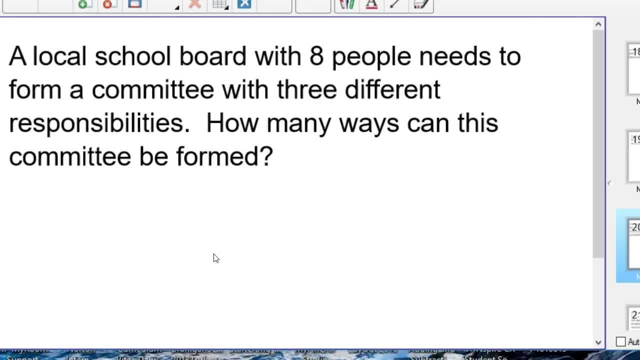 Yeah, So a local school board with eight people needs to form a committee with three different responsibilities. How many ways can this committee be formed? Obviously, this is a permutation. This is a permutation which would be eight P three. So I'm just gonna jump straight into. 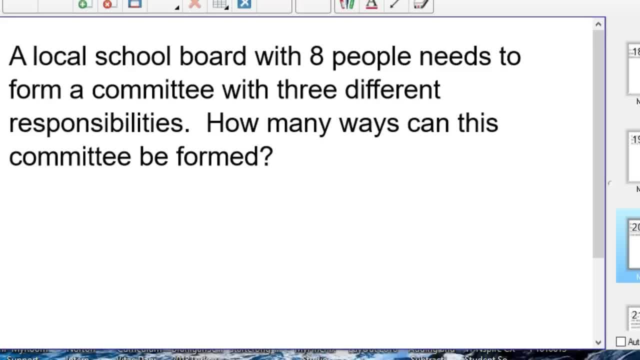 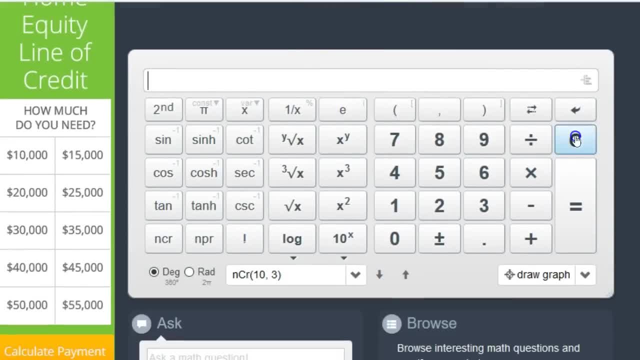 since we know it's a permutation. it would be eight times seven times six, or we could go ahead and use the Web 2.0 calculator just to show you kind of all the different possibilities. I mean, whatever you have for technology is great. 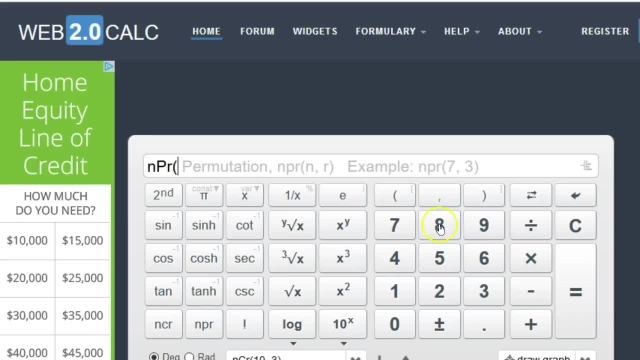 It probably does it, So I'm gonna hit permutation eight comma three Should be larger than the combination. Here's the formula: Hit equals and it's 336.. So there you have it. So let's take it up a notch. 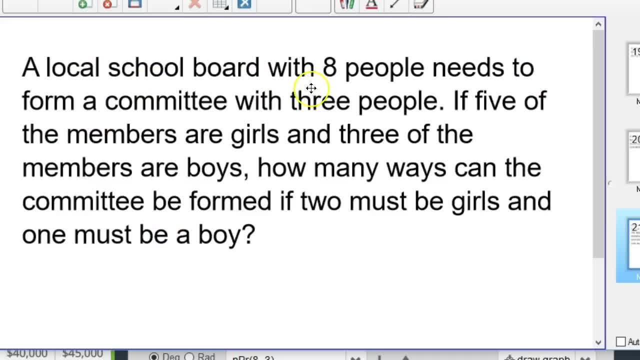 Let's say, a local school board with eight people needs to form a committee with three people. But we will throw in a twist: If five of the members are girls and three of the members are boys, how many ways can the committee be formed? if two must be girls and 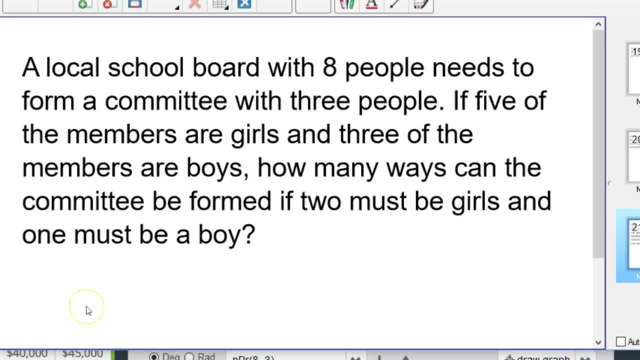 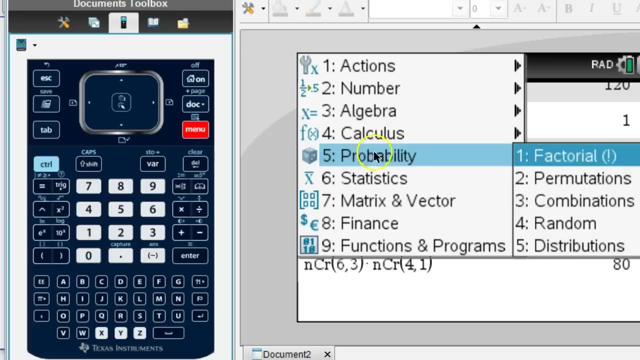 one must be a boy. So hit pause on the video and see if you can solve this. So I'll go ahead and just show you quickly on a calculator how to do this one. I've got the TI Inspire loaded up again, So you hit Menu- Probability.